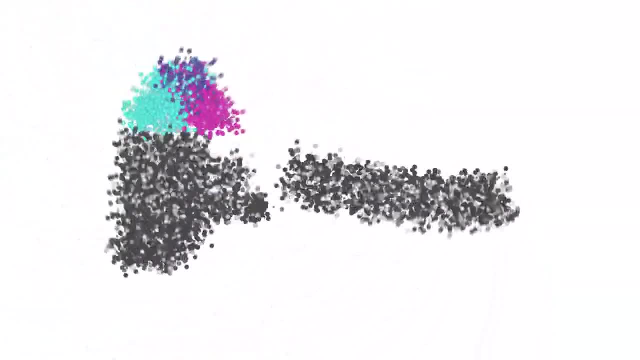 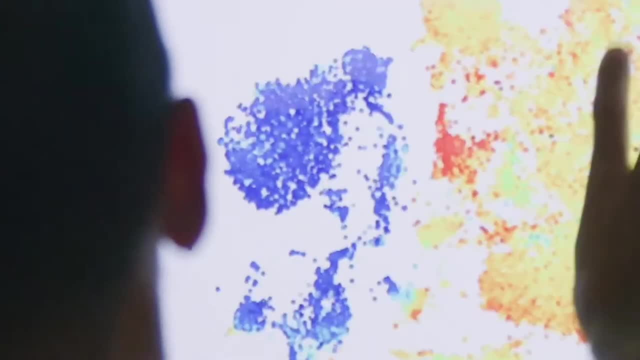 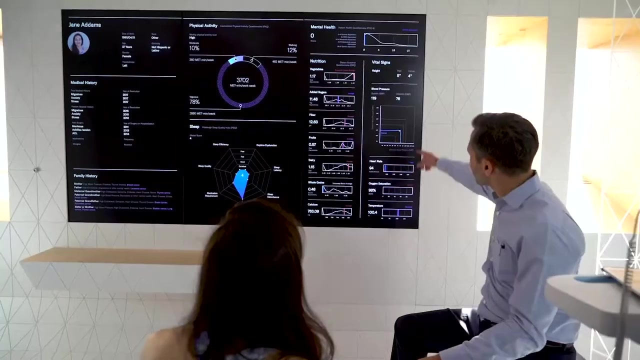 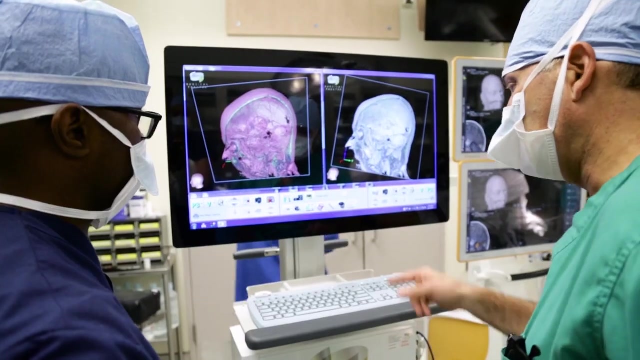 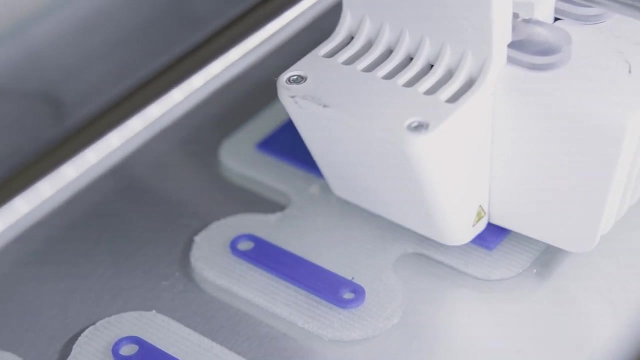 It's an exciting time to be a researcher in the fields of artificial intelligence and emerging technologies- computational biology. We're really entering a new era where technology is becoming more infused into the life sciences and into biomedicine. We're using computational powers in ways that we've never done before in biology. 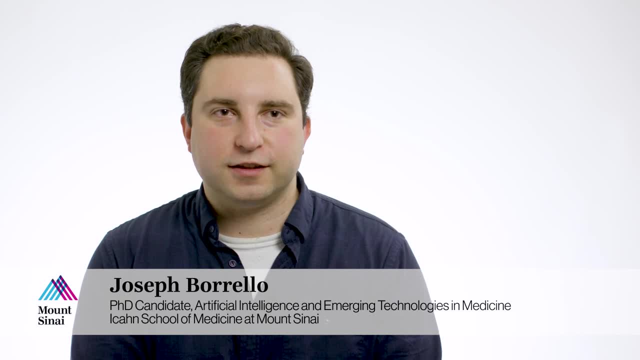 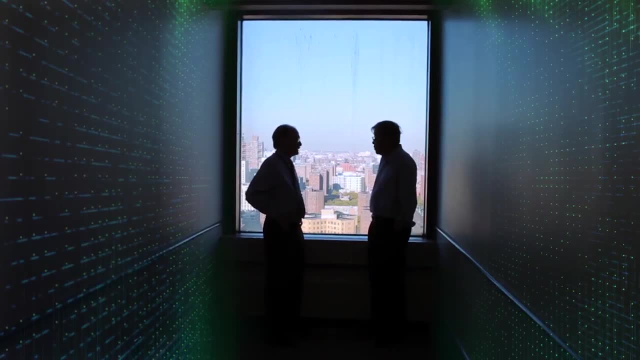 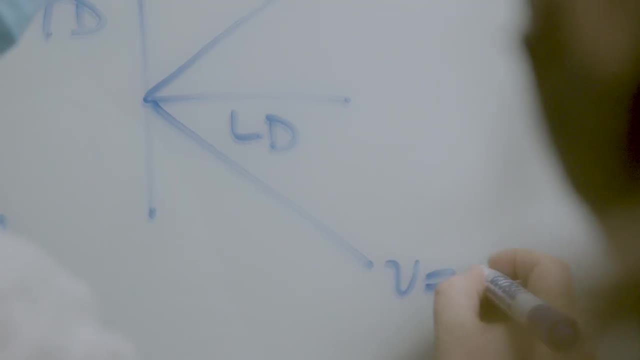 I definitely think Mount Sinai is leading the way when it comes to artificial intelligence research and the emerging technologies in medicine. The artificial intelligence and emerging technologies in medicine training area is super exciting. Creating this program will take artificial intelligence to a new level and enable students 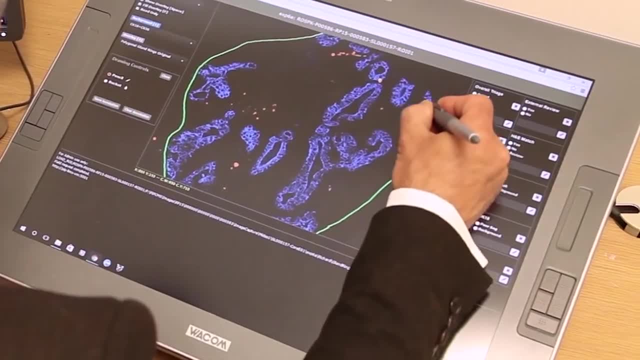 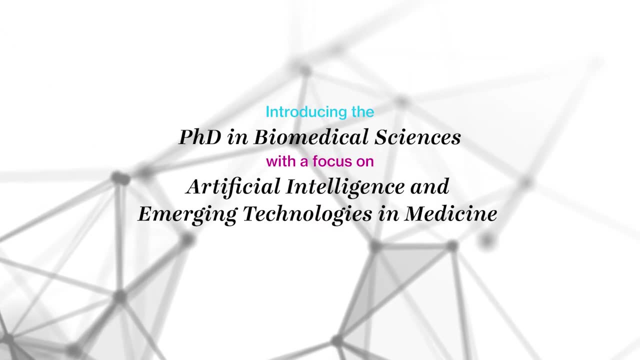 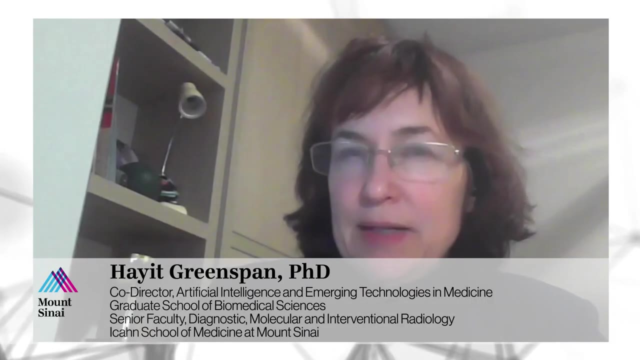 to work on projects They wouldn't have been able to previously. Once you've gone through the program, you've really seen how biomedicine and healthcare works at every level. The idea behind this program is that we want to combine computational capabilities from 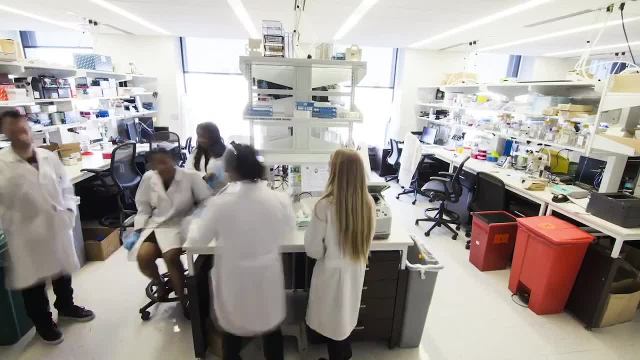 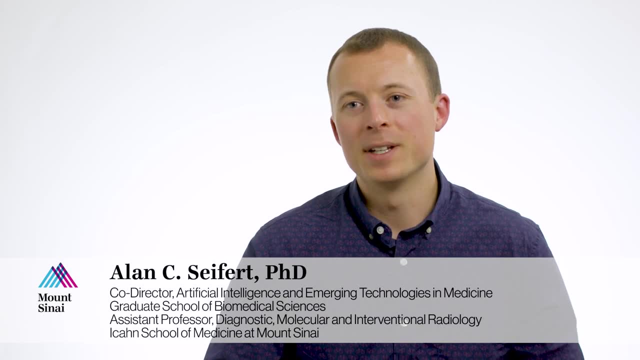 engineering and computer science applied math to the field of medical research and medicine at large. What we're creating here is the artificial intelligence and the emerging technologies in medicine. It's the environment and the opportunity for our students to directly make a difference in patient care. 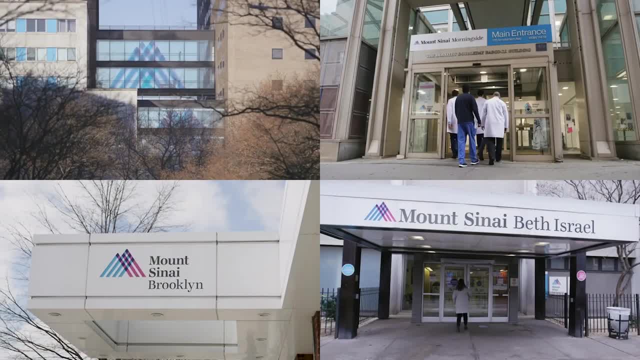 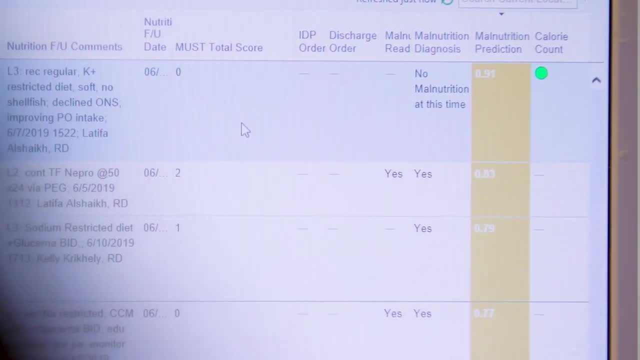 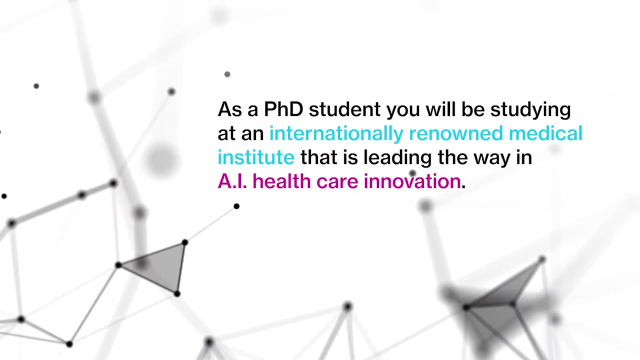 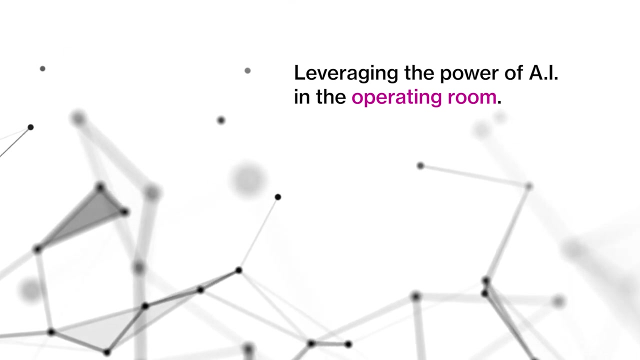 Just the sheer opportunity to work in a massive medical system with incredibly rich data sets related to all kinds of things related to patient care, and then to partner with physicians and scientists on real world problems is just tremendous for young students. What I'd like to do is direct the future application of technology on skull base and 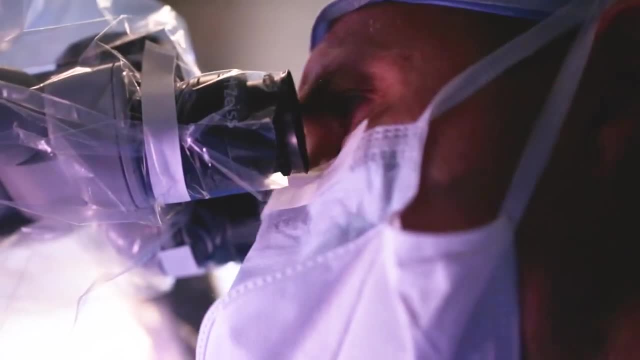 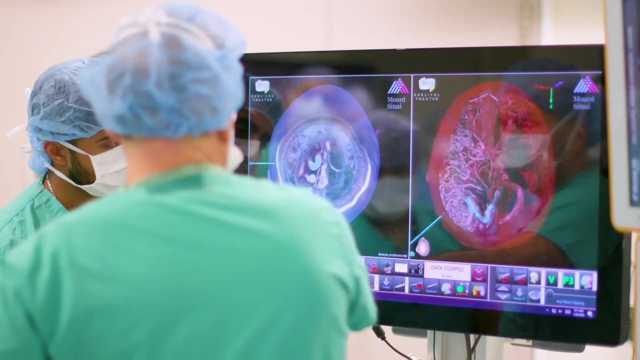 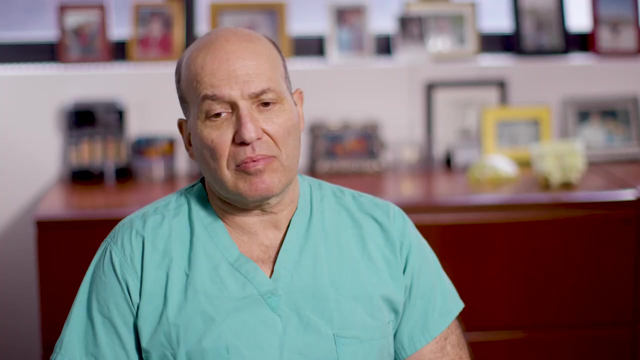 cerebrovascular surgery. The use of 3D virtual reality scenarios created for each patient based on their own anatomy and linking it to the 3D scenario we created so that I can see through tissues and see around corners in ways that were not even something we could dream up many years ago. 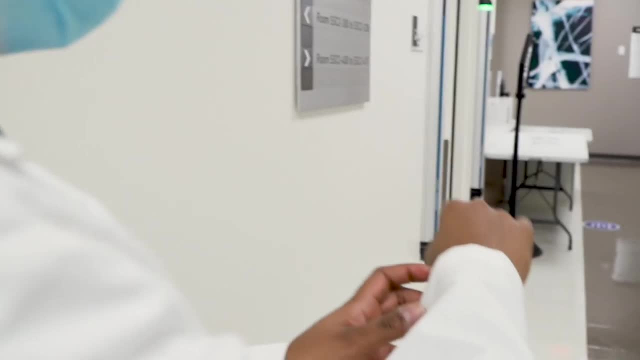 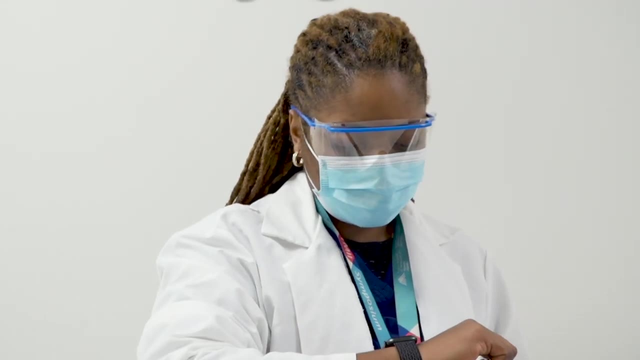 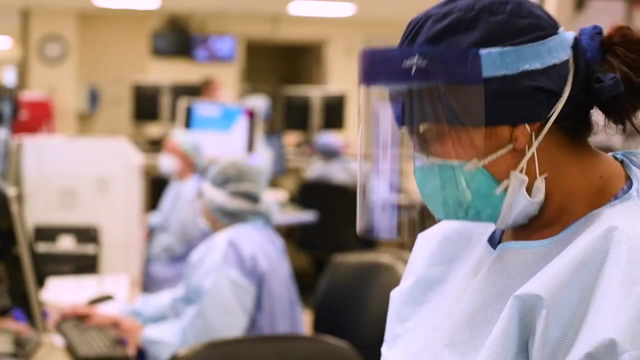 We wanted to really honor our frontline healthcare workers for what they have done during the COVID pandemic. We designed a specific app to understand better the level of anxiety and stress they are faced with, the effect of chronic stress on the brain, but also on the cardiovascular system. 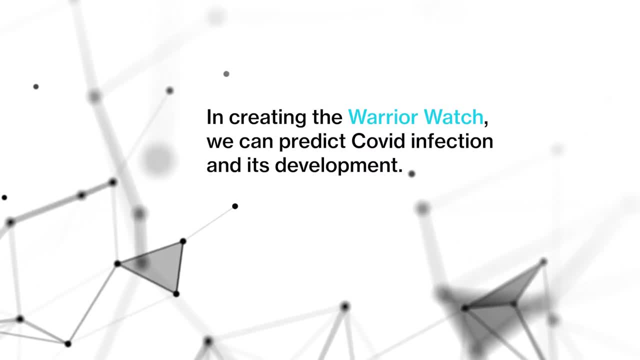 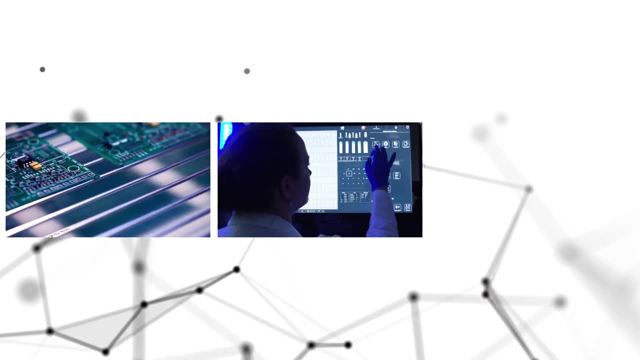 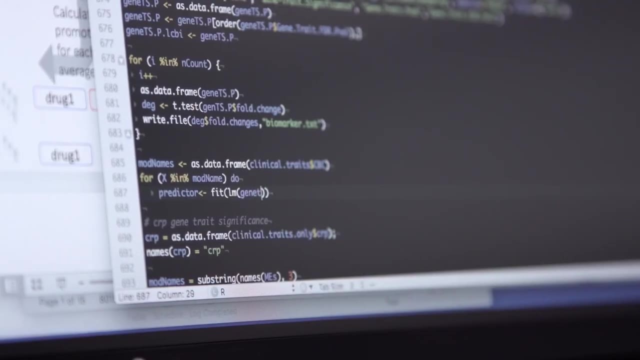 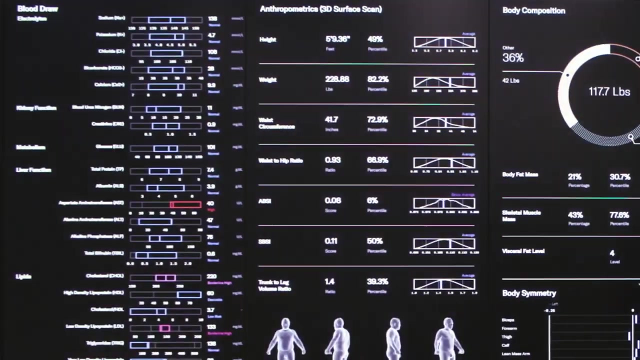 and on the immune system. Mount Sinai is bringing data science to the frontlines of healthcare. We're creating, in a very rapid fashion, tools that can make the world safer for our patients. The game changer that we're talking about is creating not just technology, but technology. 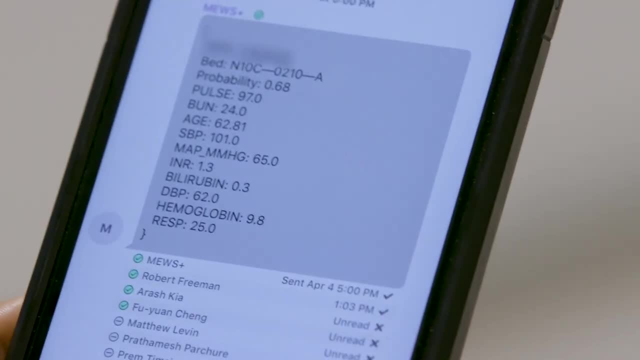 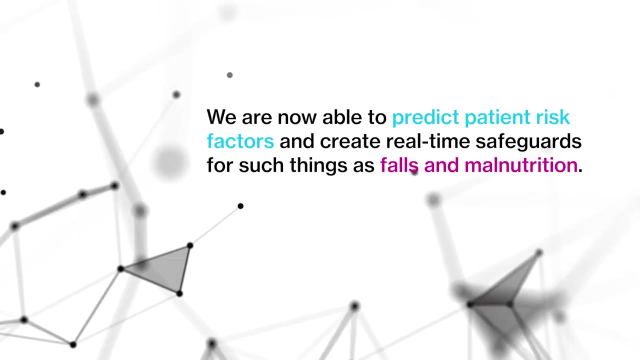 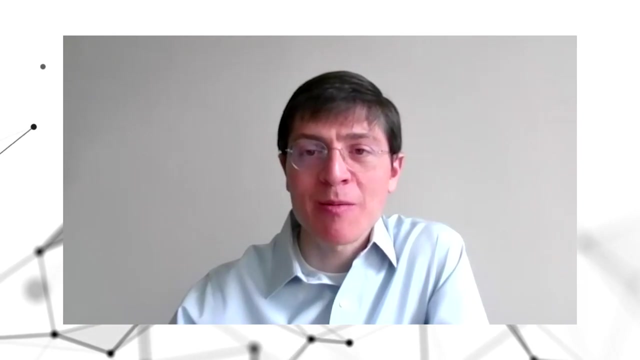 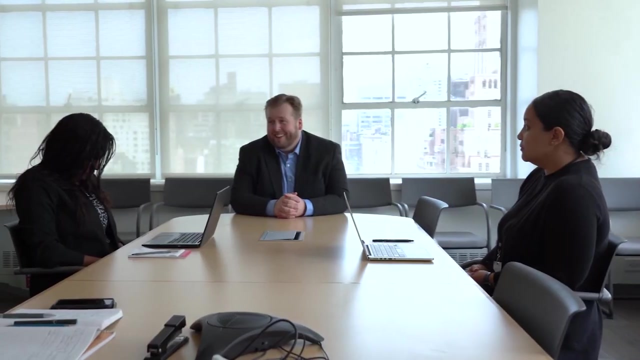 that is accessible and usable for the healthcare delivery professionals. That's the vision as we go into the future. The sky is the limit. Anywhere you look, you're going to find a place where you can do something new and creative. Within this program, we've assembled the best of the best that students are able to work with. 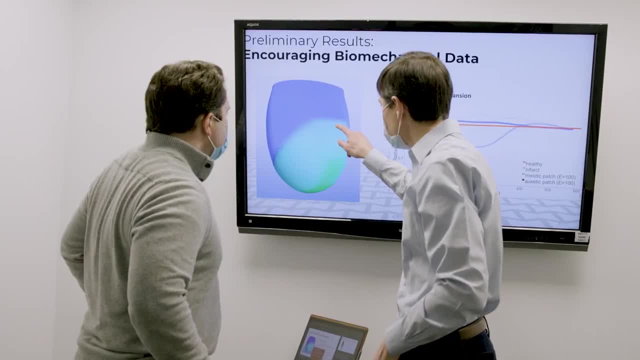 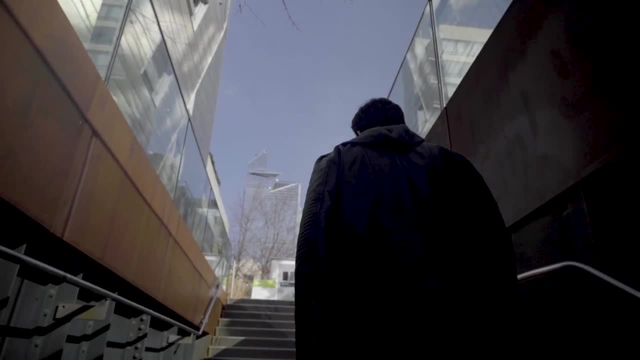 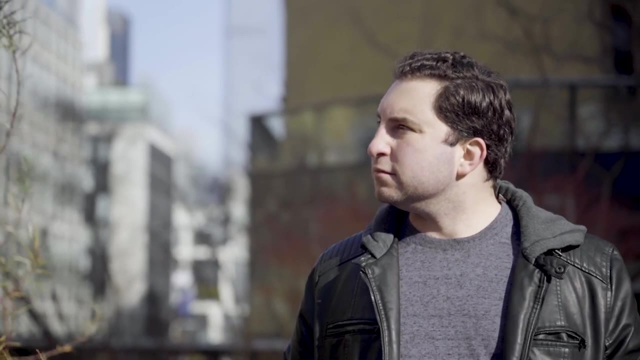 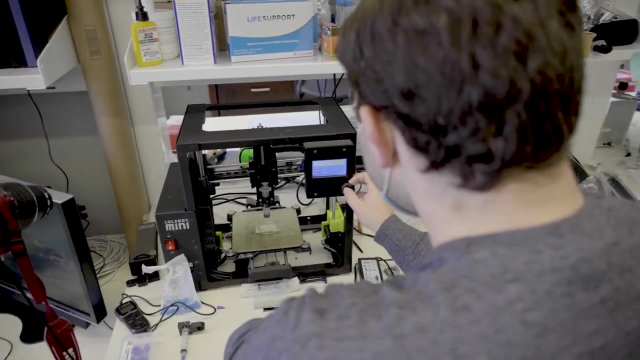 Each researcher at Mount Sinai is unique and exceptional. When I was looking for a PhD program, I was very interested in doing something entrepreneurial and innovative. I was looking for the opportunity to do research that would have a direct impact on patients and an actual, deliverable outcome, some kind of physical thing that we could produce and 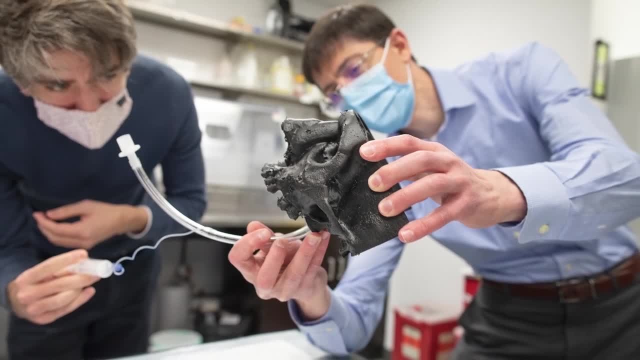 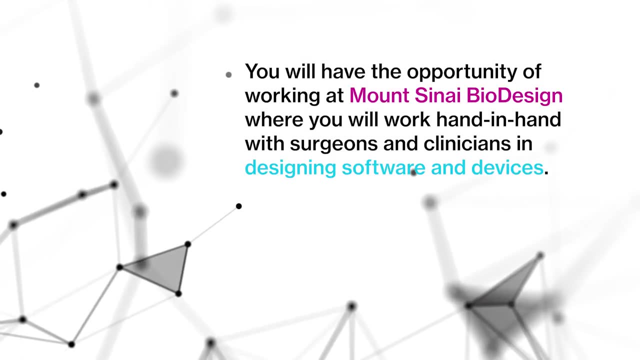 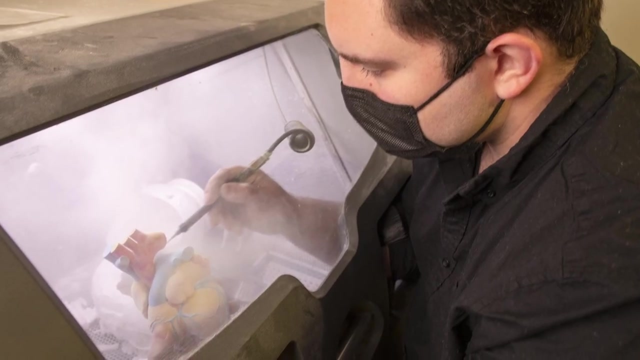 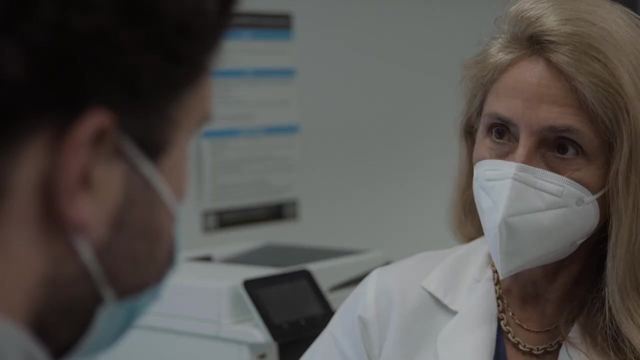 say: we made this. Our students will be able to create new technologies and new methods that they can test in a clinical setting. My research focuses on developing mechanical metamaterials that can replace native tissue in the body, And artificial intelligence and advanced computational design offer new opportunities to create. 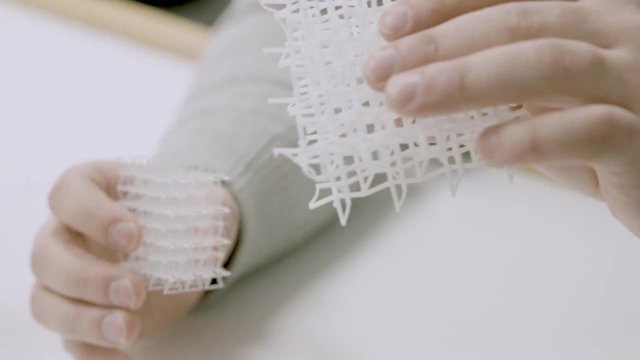 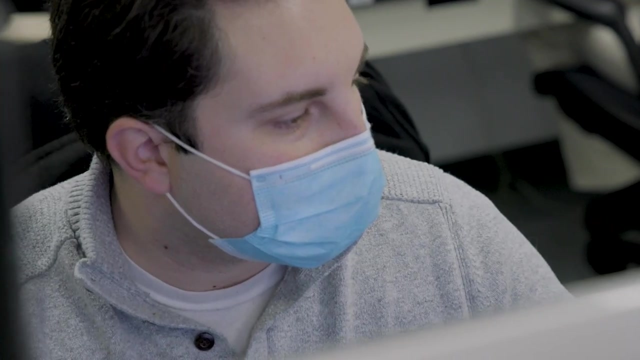 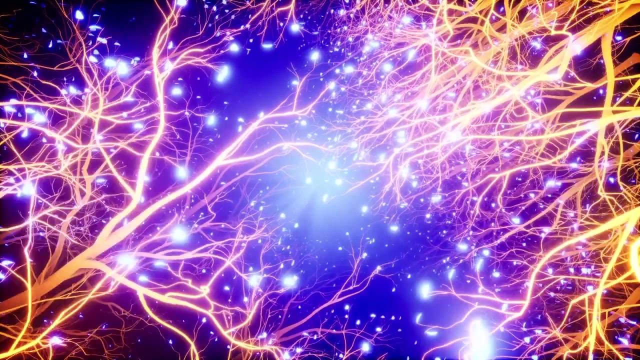 materials that can be structured and manufactured in different ways and will better meet the applications that they need in the human body. We have PhD students who are working on automated techniques for interpreting medical imaging. We have PhD students working on sensors and artificial intelligence applications in medical 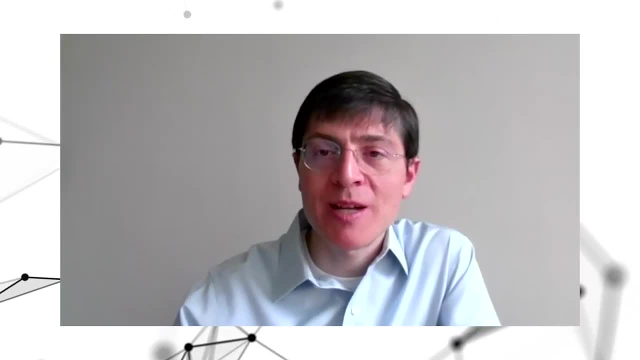 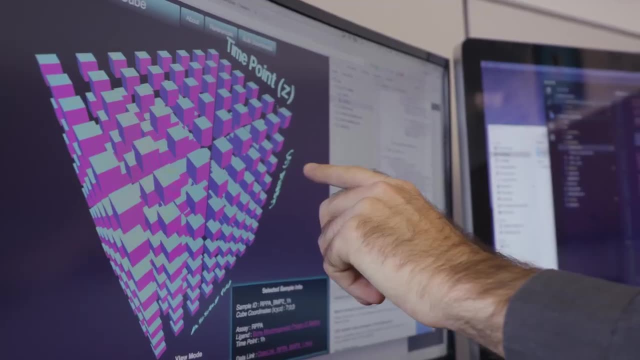 imaging. We have a PhD student who's working on artificial intelligence for the medical imaging. We have a PhD student who's working on artificial intelligence applications in surgical robotics. When you're here at a place like Mount Sinai doing cool, innovative work, you're basically